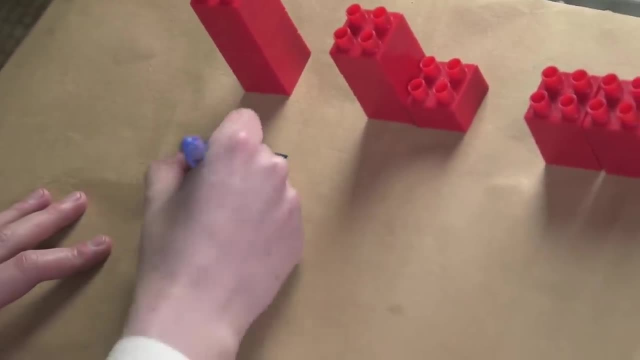 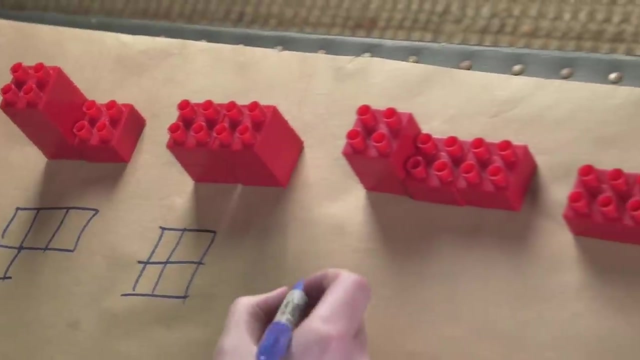 So if we draw this out, we can either draw it like this: 1, 2,, 3, 4.. We can do a 3 and a 1,, like that: 2, 2.. We could have 2, 1, 1.. 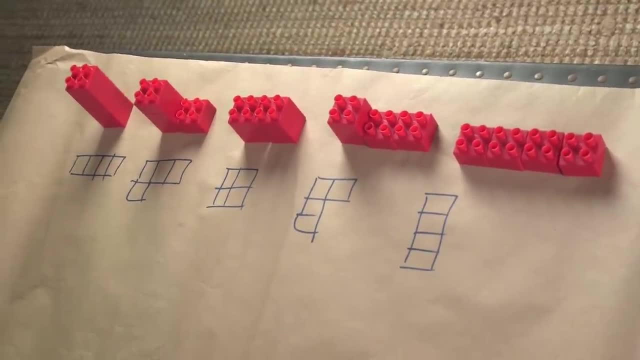 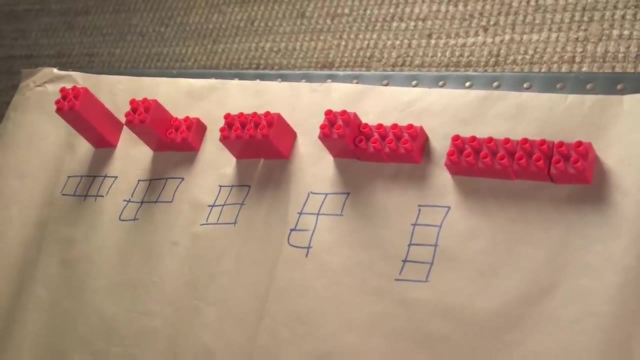 1, 1,, 1, 1, like that. So this is what mathematicians actually do. They do it this way because by seeing it as a picture, you can actually make conclusions about partitions which are easier to see. 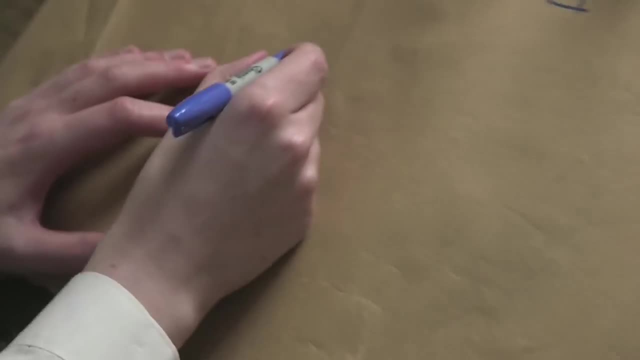 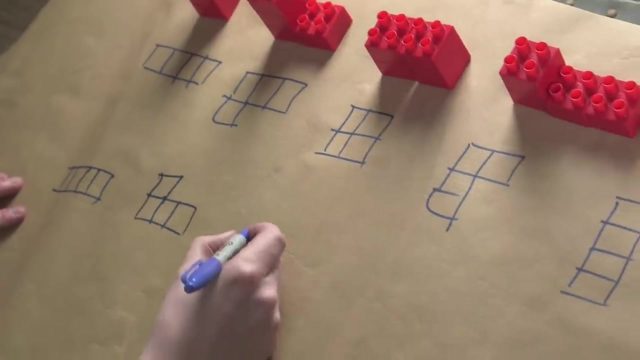 The French do this slightly differently. The French draw them like this: You can have a row of 4 like that, And you can have a row of 3 with a row of 1 like that, So slightly the other way around. Or you could do it like this: 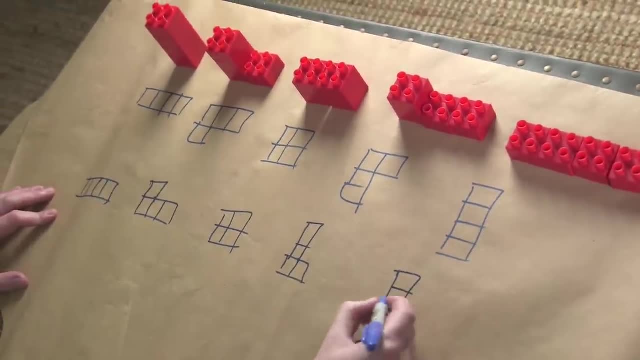 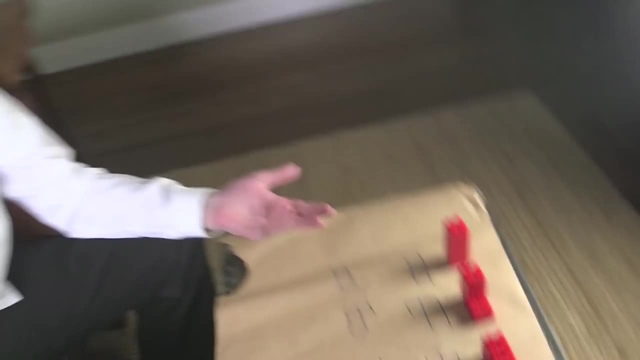 Bom, bom. And then the last one here: 1, 1, 1, 1.. So it's a slightly different way of doing it. My favorite footnote from a textbook. Do you have a favorite footnote from a textbook? Oh no, I do. 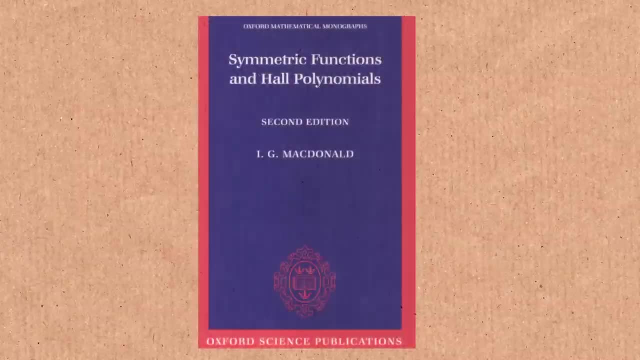 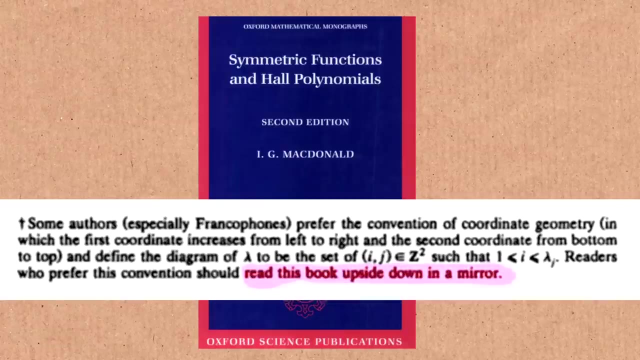 A favorite footnote from a textbook was by Ian MacDonald, who said: if you want to do the French notation, you should read this textbook while looking upside down and in a mirror. So I get to say this for myself for the first time: If you want to use the French notation, watch this video upside down and in a mirror. So let's look at the sequence of partitions. So the sequence is this: 1,, 2,, 3.. 3,, 5,, 7,, 11,, 15,, 22,, 30,, 42, and so on, like this: 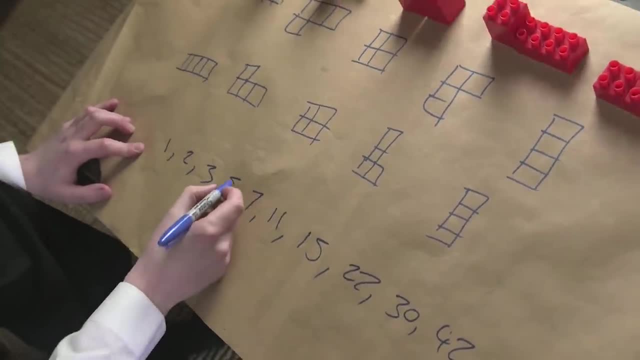 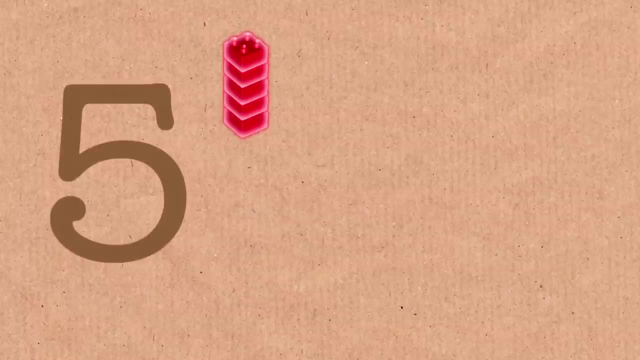 OK, so when we were looking at partitions of 4, that's this one- here There are 5 partitions of 4.. So if that's breaking down the number 4, there are 5 ways of doing it. If you wanted to break down the number 5, there'd be 7 ways of doing it, and so on. 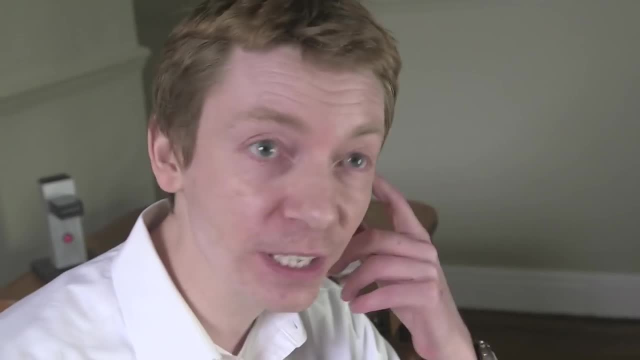 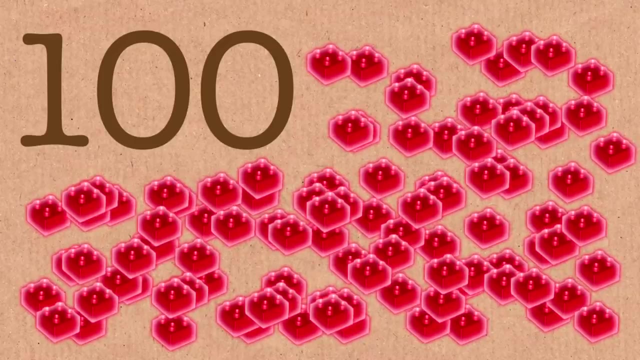 So these numbers get larger And by the time we get to something like 100, right, how many ways could we break down the number 100?? If we did that, it's going to be a lot. It's going to be a large number. 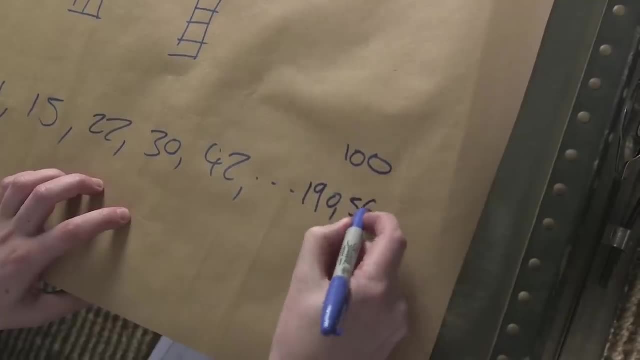 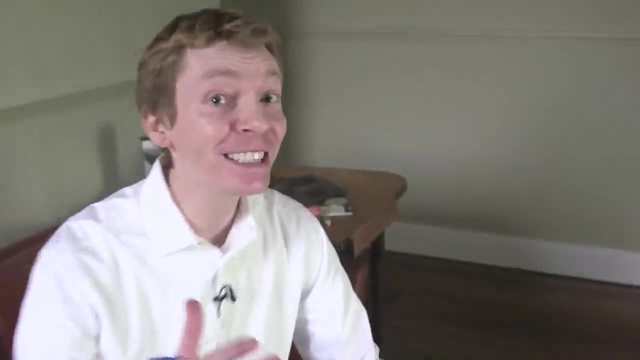 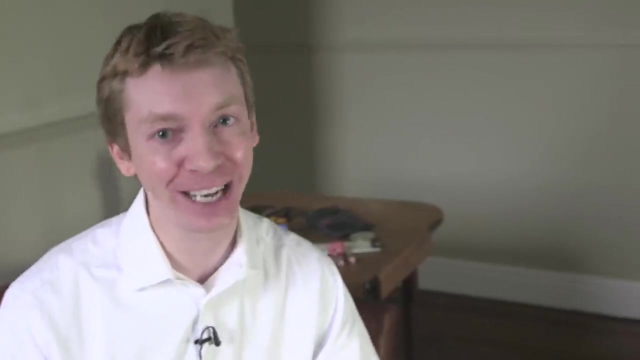 It's going to be 190,569,292.. So these get really large. Now it becomes very difficult to calculate these partitions by hand. Wouldn't it be nice to have a formula that helps us work out these partitions? So then, if I have a formula, you can give me a number. 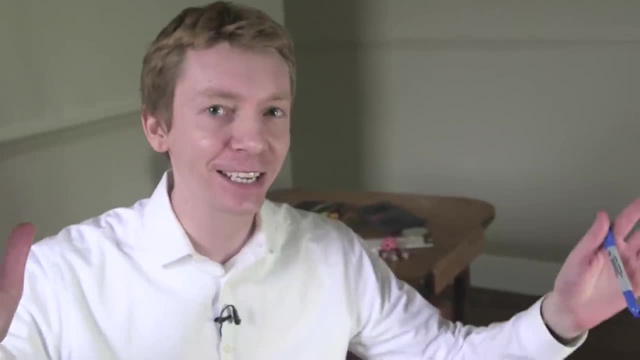 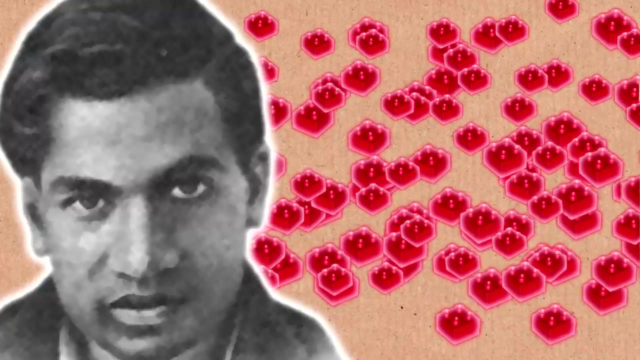 and I can tell you how many ways to break that down. Oh, fantastic, And this is the problem that Ramanujan decided to tackle. So there were some formulas before Ramanujan which go back to Euler, Not particularly pretty formulas, but I could show you what they look like. 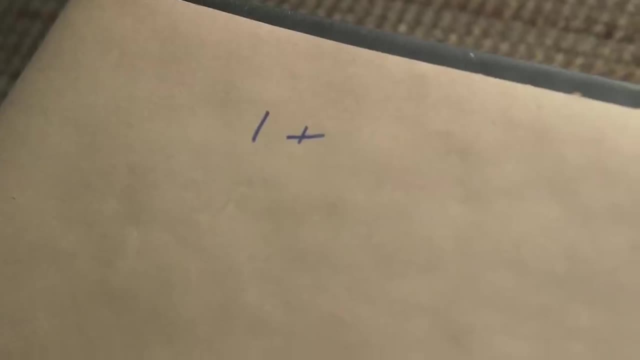 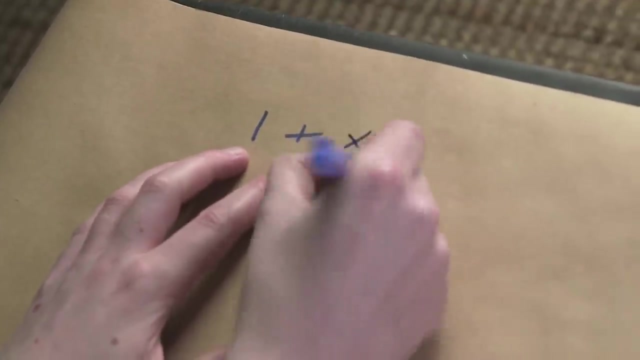 Shall, I do that. Okay, so I'm going to draw out a polynomial using partitions as coefficients. It means it's going to look like this: 1 plus. I'm going to have plus, x, plus. Now I'm going to have x squared next. 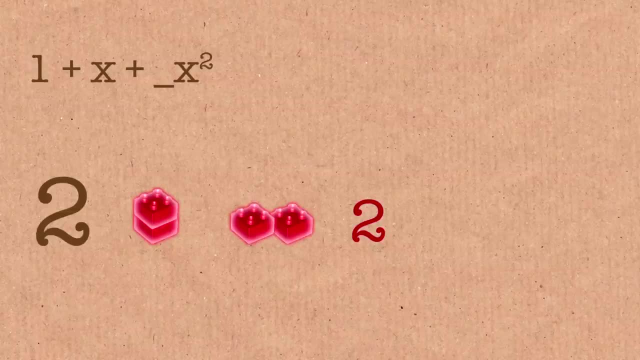 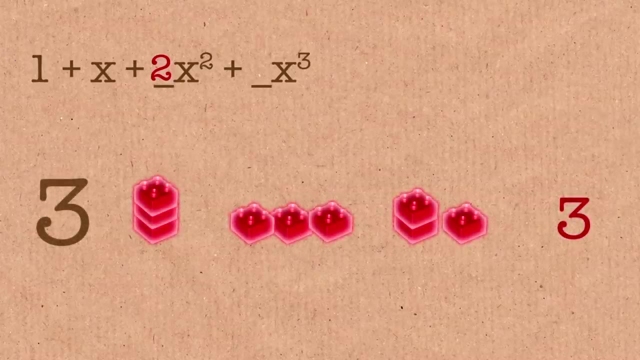 but I'm going to use how many ways to break down 2 there, which is two ways of doing that. So if I had x cubed, next how many ways to break down 3? And there are three ways of doing that. 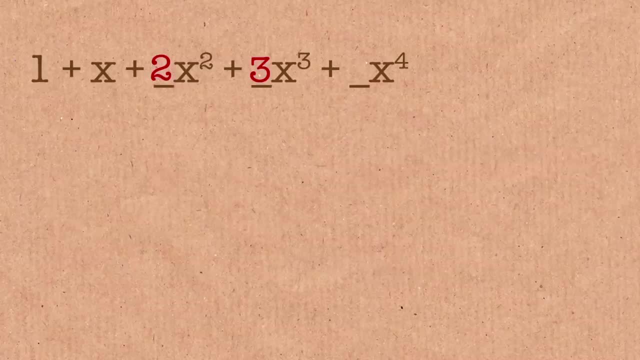 And now I keep going like this. So if I had x4, we know how many ways to break that down right. There are five ways of doing it, And then it's 7 for x5, and so on, like this. 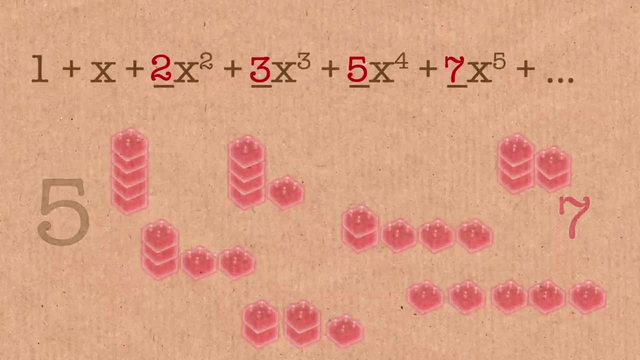 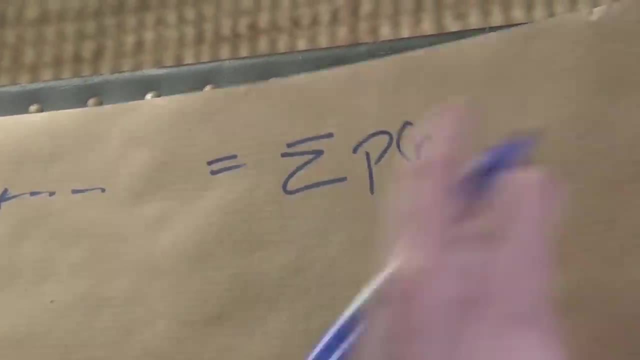 So this is a very maths-y looking thing. In other words, if you like this notation, which means sum, if I want a sum, these are called partitions of n, and then it's times x to the power n. There you go. 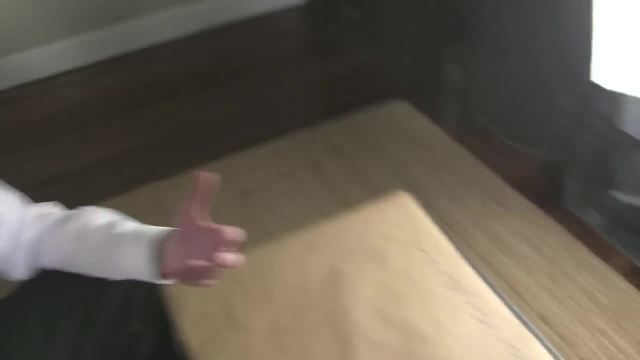 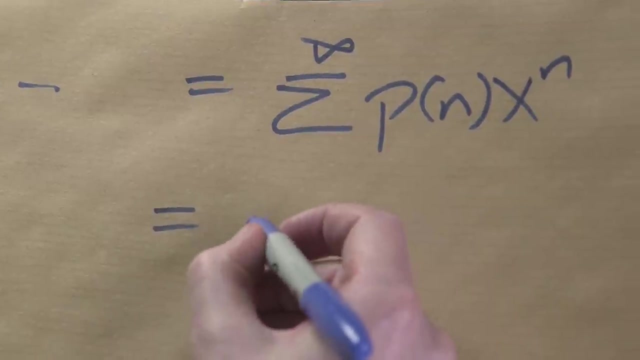 And you do that all the way up, All the way up to infinity. Now, what Euler saw was: this was equal to. This is equal to. I'm going to use another symbol here. This symbol, which is a capital, pi, means product. 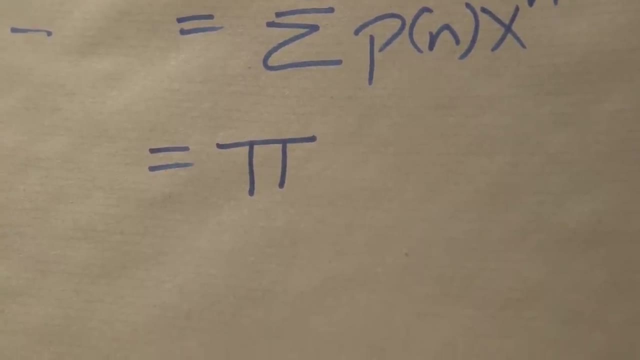 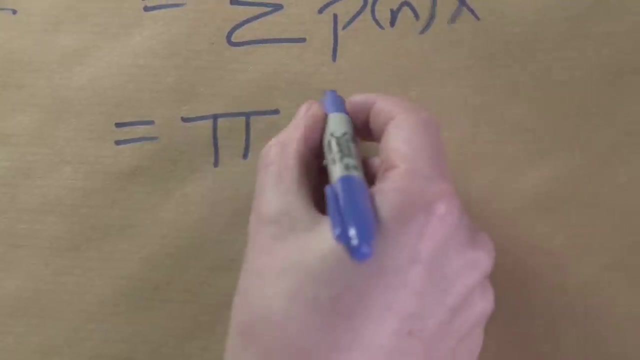 It means you're multiplying these things together, Not 3.14.. It's not 3.14.. Yeah, we're limited to how many letters we've got to use, So we're using pi here for product, The product of 1 over 1 minus x to the k. 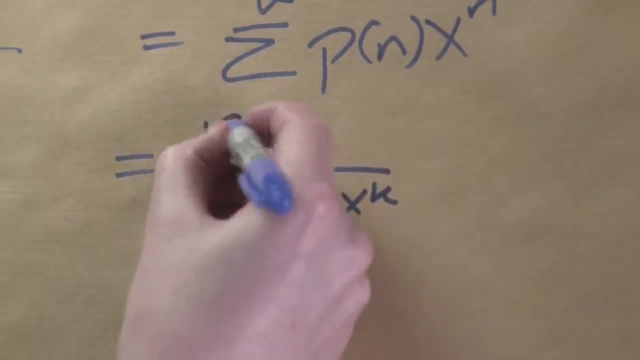 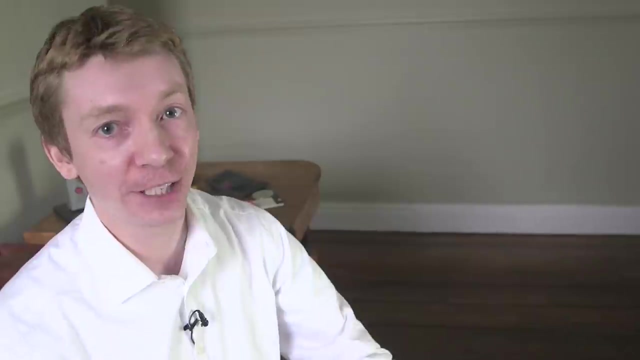 There we go. We've got this is from: k equals 1 to infinity. So we've got something that we're multiplying together. It's equal to this polynomial. So this is a way of working out partitions And this is what you used to do classically. 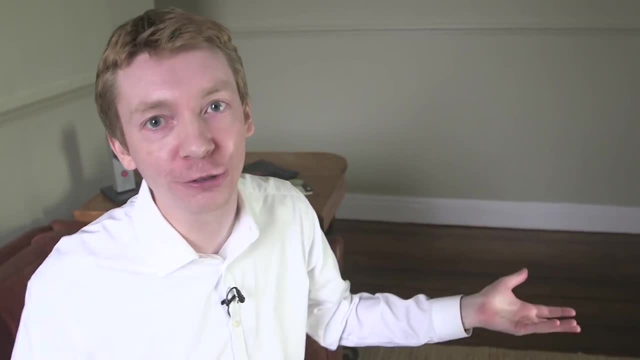 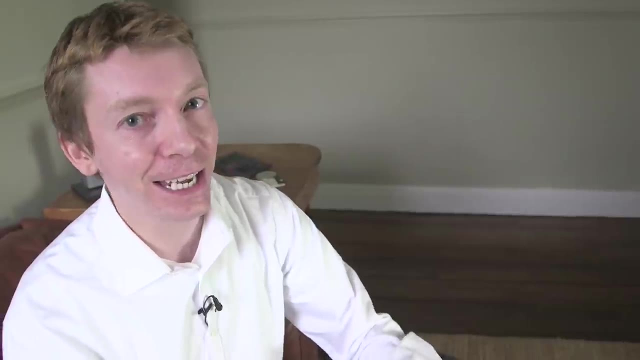 And so if you want to work out the partitions of 100, you could use a formula like this and actually do the calculation, But it's not particularly easy, But that is what they used to do if they had to do it by hand. 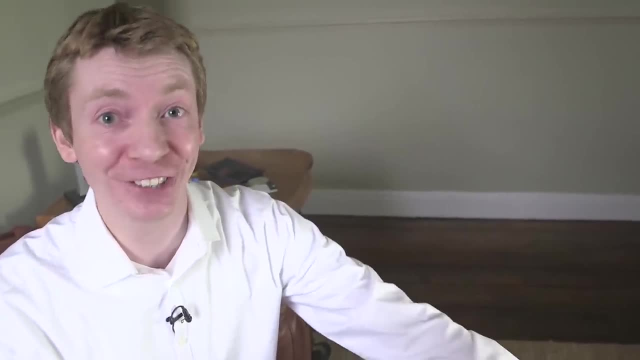 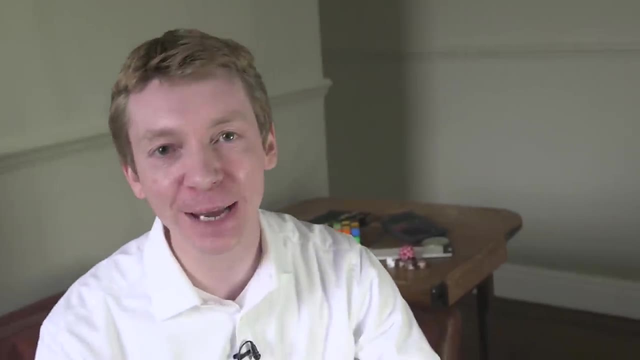 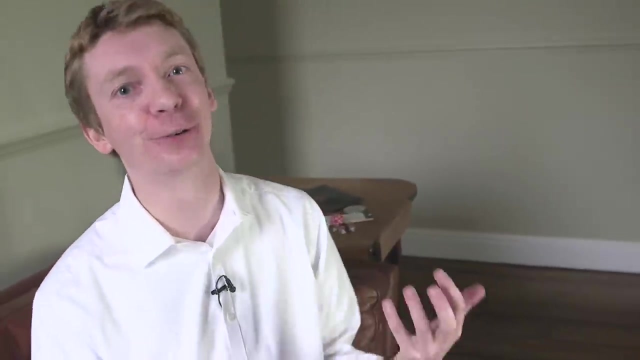 And it's what your computer would do. if it wants to work out partitions, It would use a formula Like that. Ramanujan had an amazing intuition for numbers. Another Cambridge mathematician called John Littlewood said that all the positive integers were Ramanujan's personal friends. 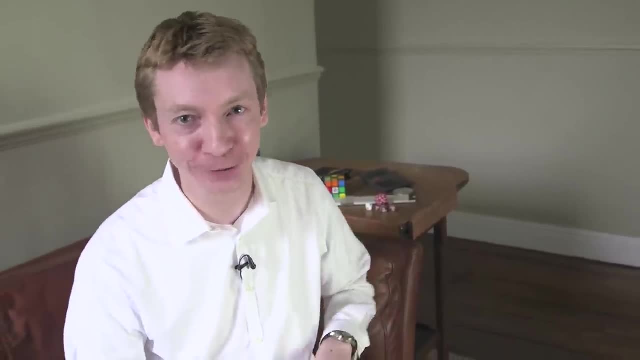 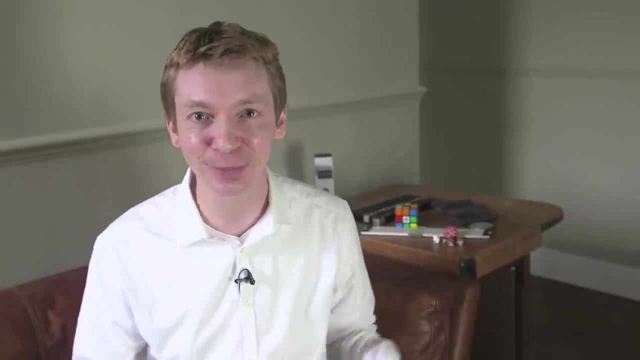 Which sounds like another nightmare to me. Having infinitely many personal friends, Imagine the Christmas card list Sounds terrible. So let's have a look at some of the things he noticed about partitions. I guess this is something that attracted him to the subject. 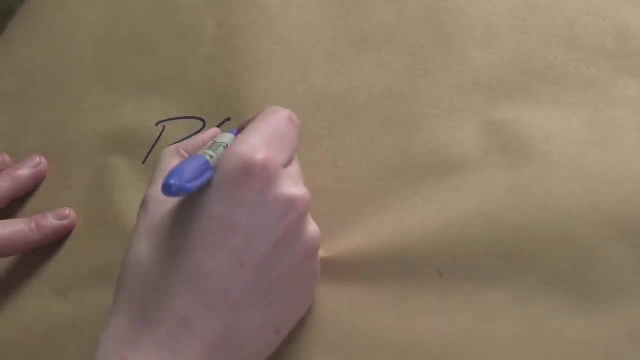 We're looking at partitions of, let's say, a number, A number that looks like this: 5k plus 4.. Okay, So if you have a number like that, it ends with a 4 or a 9.. 4,, 9,, 14,, 19.. 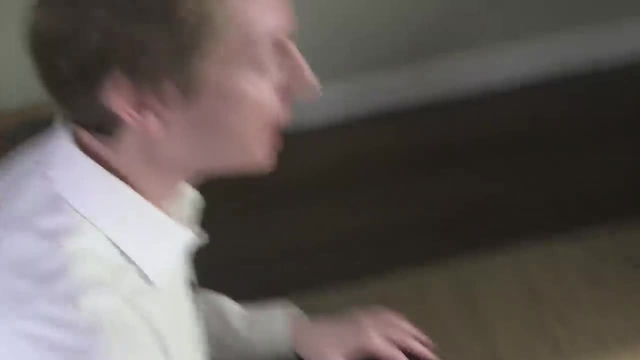 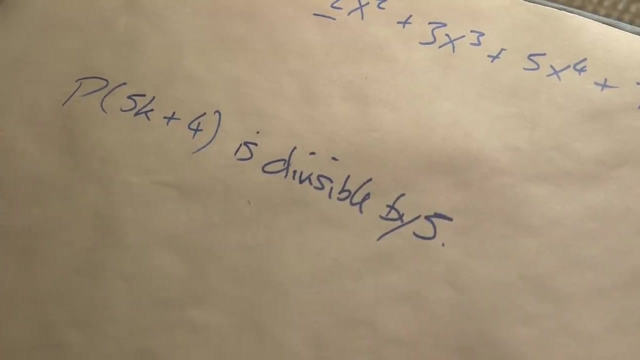 So these numbers? So if you have a number like that, he noticed something. He noticed that the number of ways of breaking it down is divisible by 5. So there's a fact that he noticed. So if you did, Let's do it. 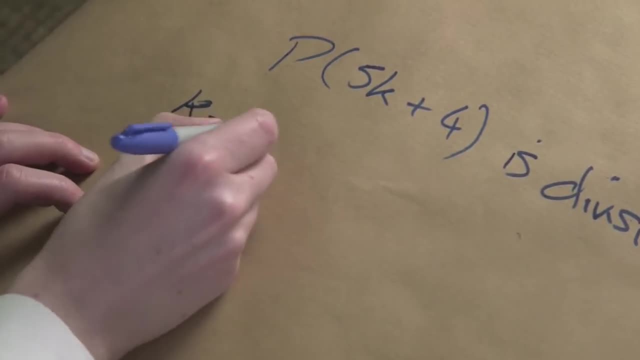 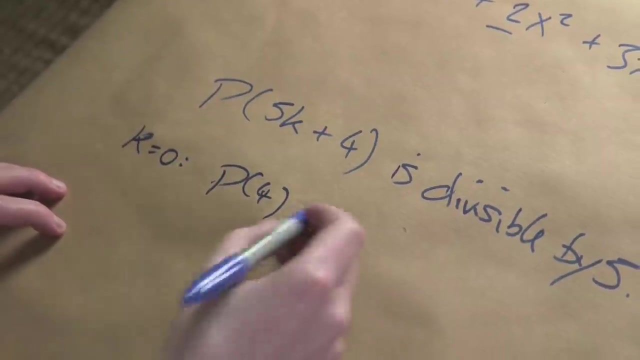 So we took the first example. So we took: k equals 0. We're looking at if it's 0, we're looking at partitions of 4.. Hey, we did that Right. How many ways were there to do it? 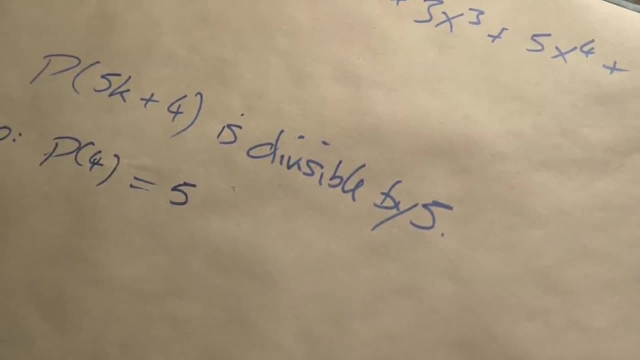 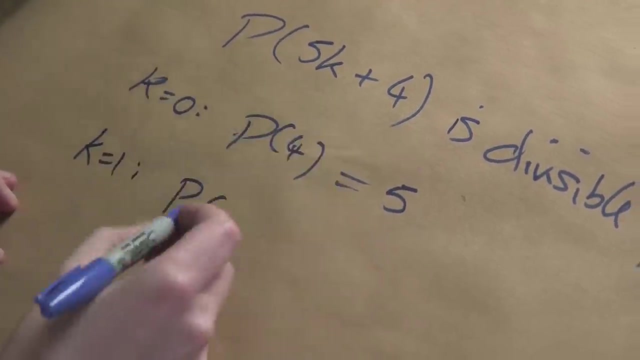 It was 5 ways of doing it. It's divisible by 5.. Great. What about partitions of 9?? So if you have k equals 1, this would be partitions of 9.. That's the next step up. How many ways of doing that. 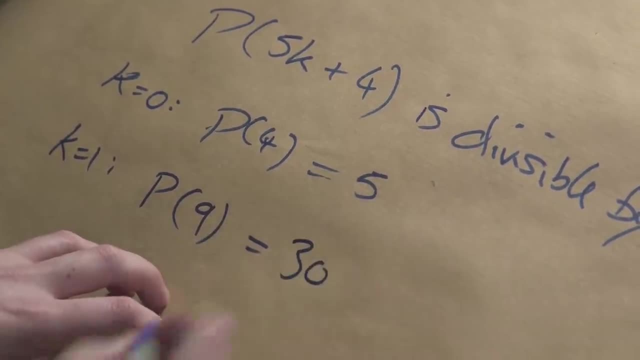 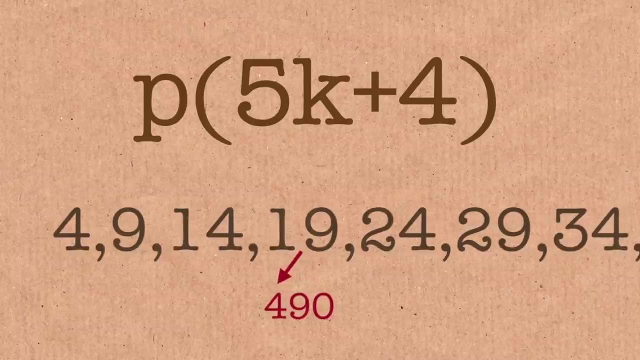 And if you work it out, I can tell you there are 30 ways of doing that. And hey, again it works. It's divisible, It's divisible by 5. And it always appears to be the case. Ramanujan was able to show this. 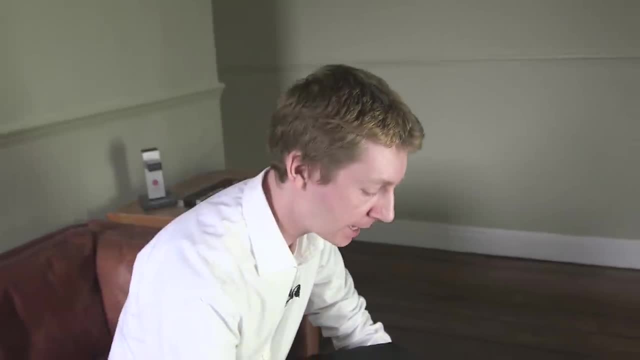 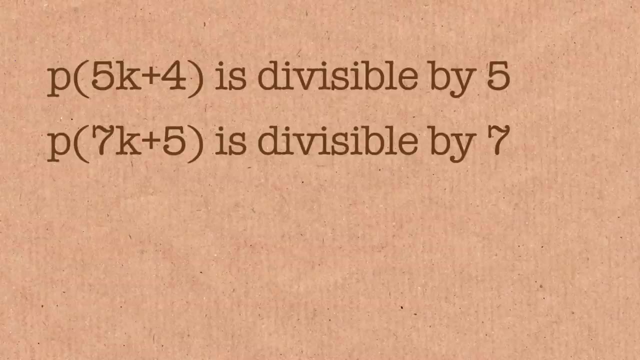 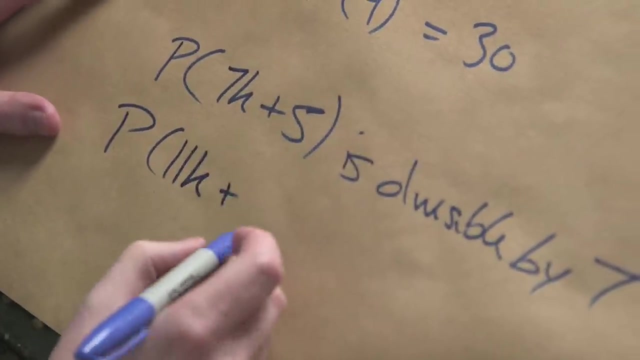 And then he was able to show a couple of things that were similar to this as well, Like if you had partitions of a number that looked like this: 7k plus 5,, then that is divisible by 7.. Or if you had partitions that looked like this: 11k plus 6,. 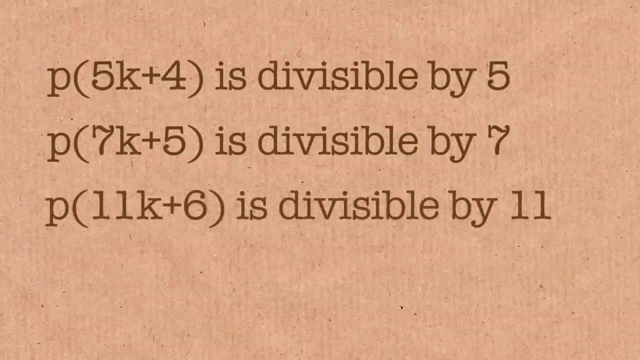 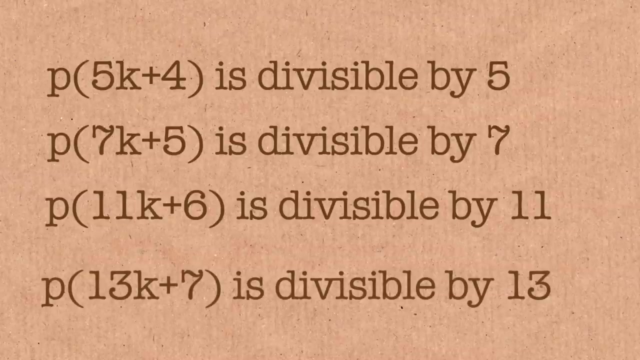 then this is divisible by 11.. We had these little facts And if you see that pattern, it does look like this. It does seem to appear like the next one should be something like this: Partitions of 13k plus 7 is divisible by 13.. 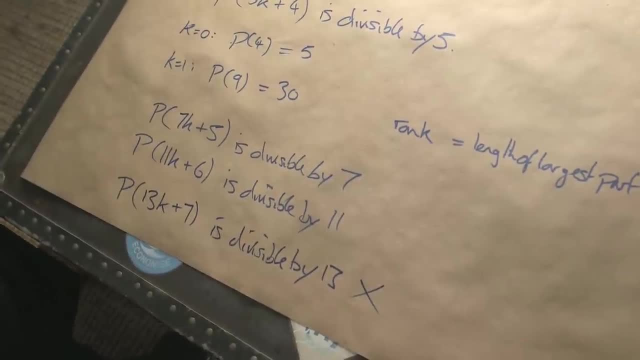 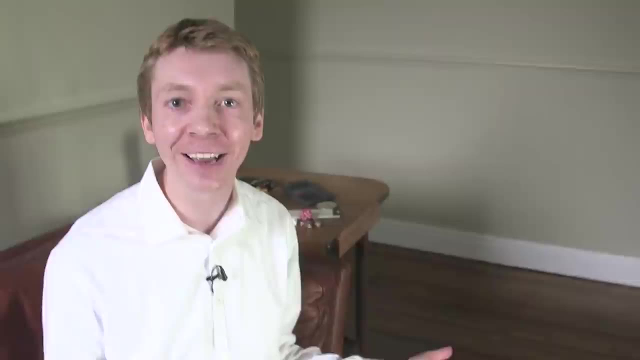 And that is not right. That is incorrect. The pattern doesn't hold. Ramanujan found these three and they found no other formula like this And they thought: well, that's it. Those are the only formulas we've got. 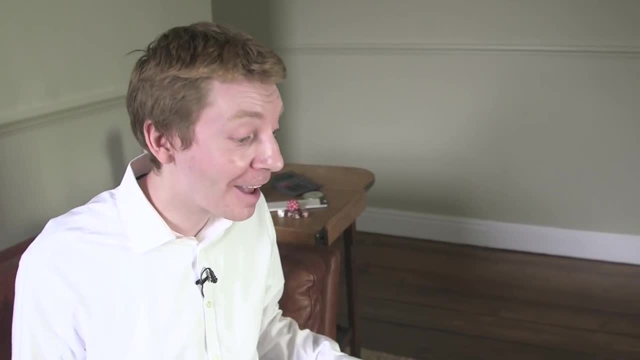 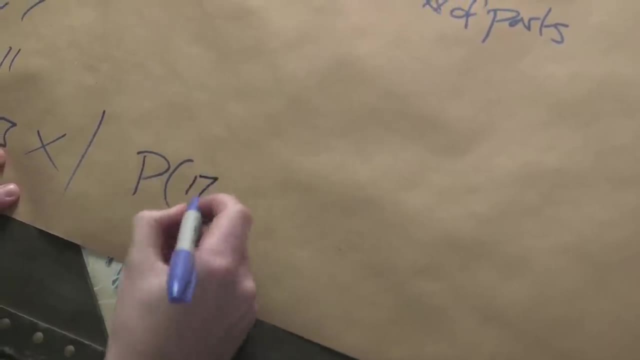 I mean the next one doesn't hold, The others don't appear to hold. Eventually, 50 years later, they did solve this. There is one that looks like this: It's not as simple as what they thought. 17,303k plus 237 is divisible by 13,. 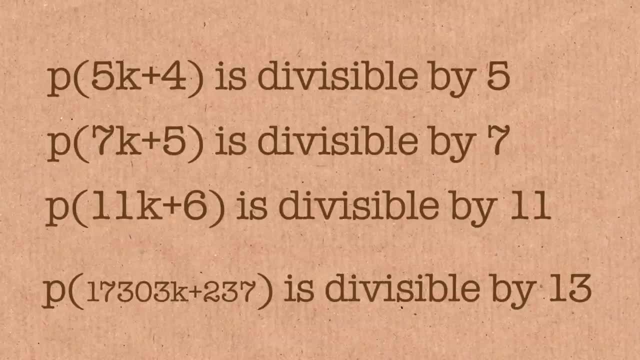 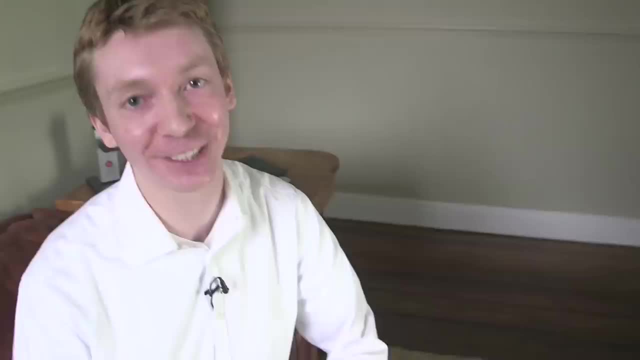 which is nothing like what Ramanujan found before. I know it seems crazy, but now we know that we have a formula like this for every prime, But they're just not as nice as the first three that was found by Ramanujan. 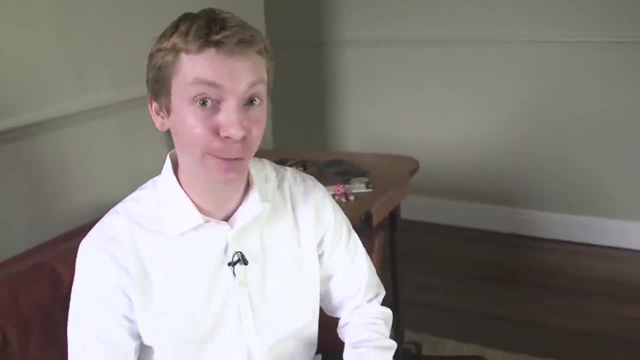 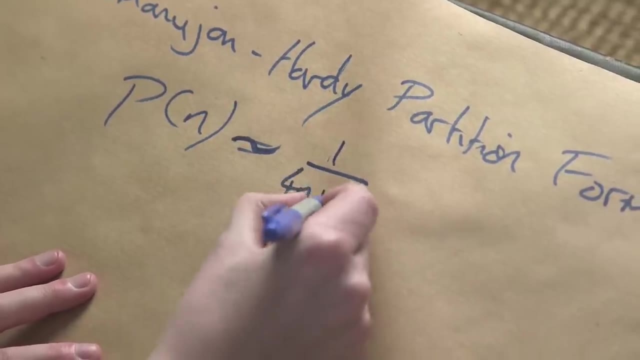 But this is still not the big formula that they wanted to find. Let's have a look at the big formula, The main punchline, Okay, Number of partitions is 1 over 4n square root of 3 multiplied by the exponential of pi. 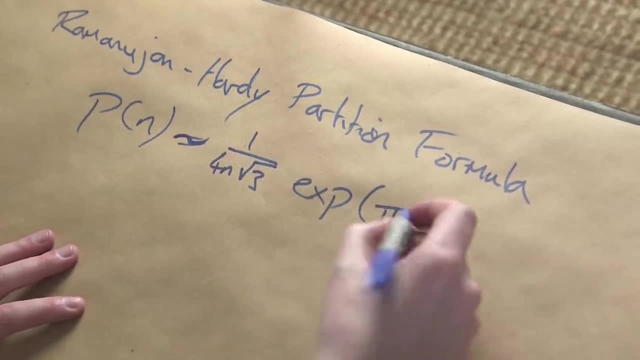 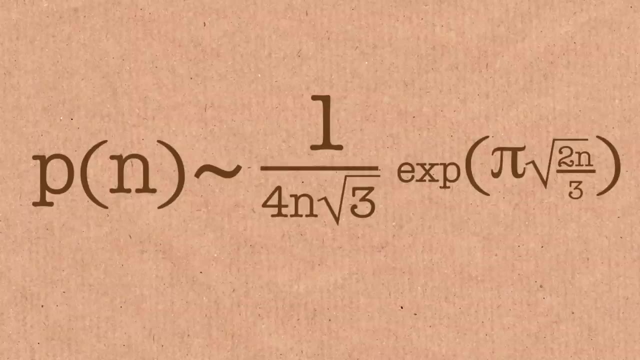 That's your traditional pi. That's 3.14 times the square root of 2n over 3.. So it's a nice closed formula for how many partitions there are. That twiddle sign, if you notice, means it's not equals. 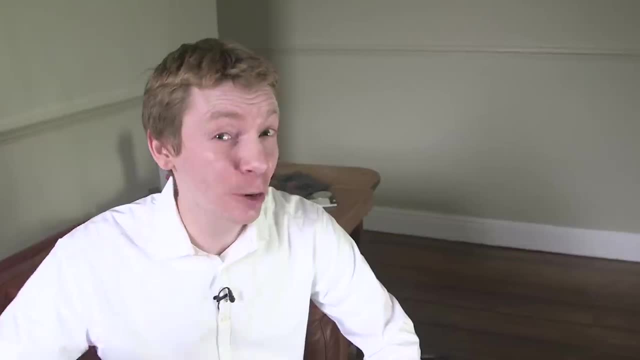 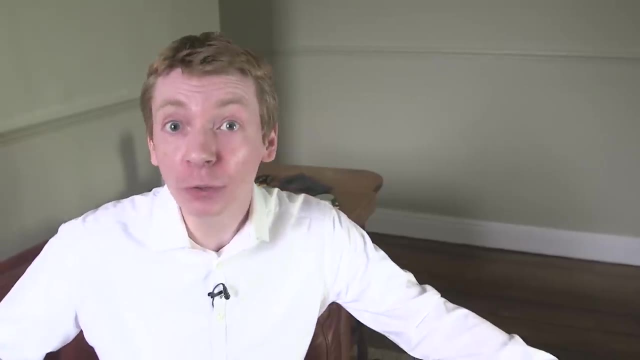 It means it's an approximation, but it's an approximation that gets better with larger values. So this is actually getting better and better as you go along the sequence. So if we did this with an example, Let's do 100, right. 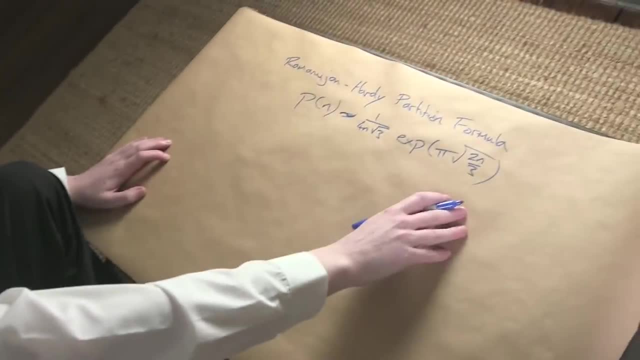 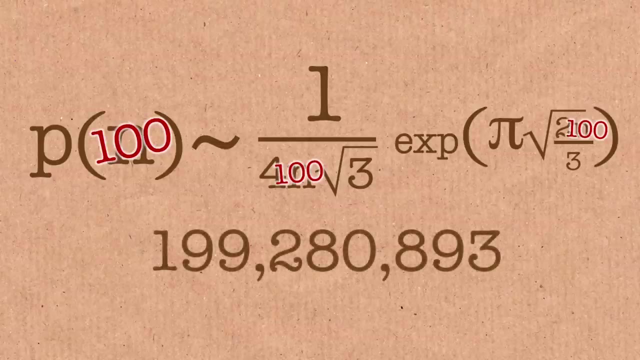 We know what the 100 value was, And if we did this with 100, if we put 100 in here, we would get 199,280,893.. Now, this is in the right area for the true value, but it's about 4.6% off. 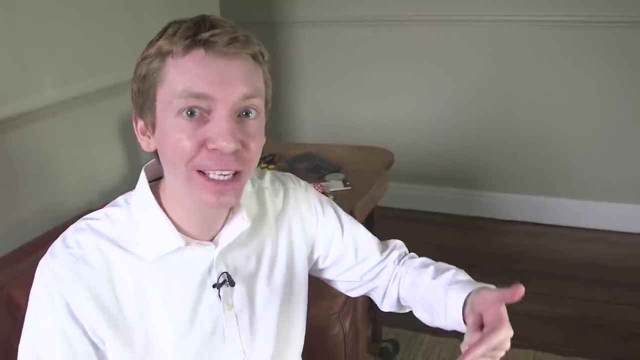 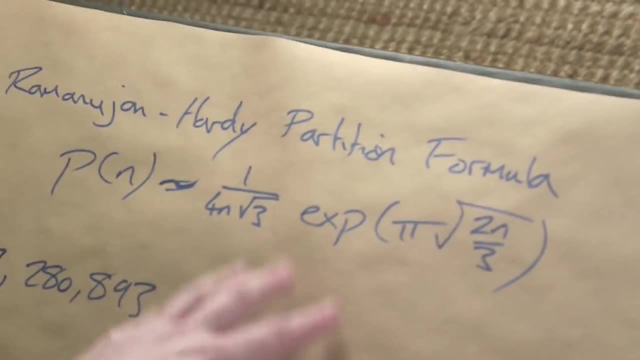 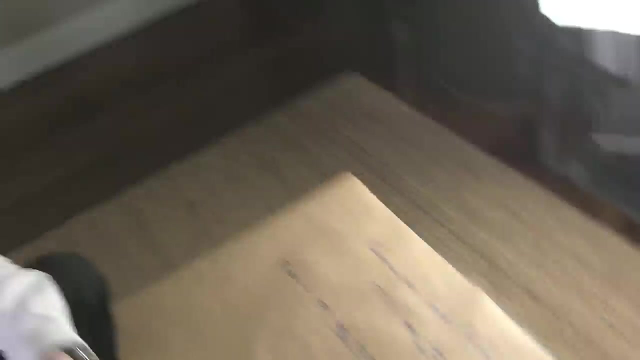 Maybe it's not the best, But again, this formula is getting better with larger values. but I can do better than that, because this formula I gave you here is actually just the first term in a series, So this can actually become more accurate. 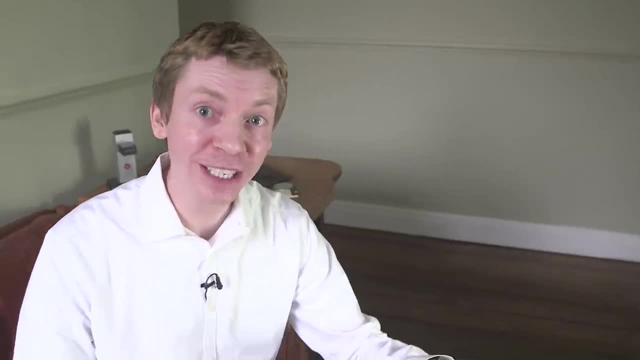 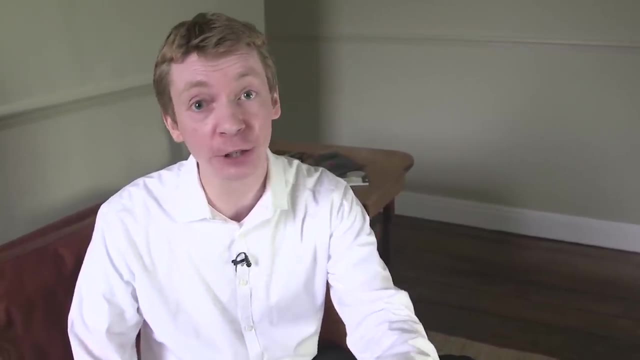 In fact it becomes equals. So what Ramanujan was able to do was use his full formula, and he just needed the first five terms to work out the value for partitions of 200 to the nearest integer, And you can do that. 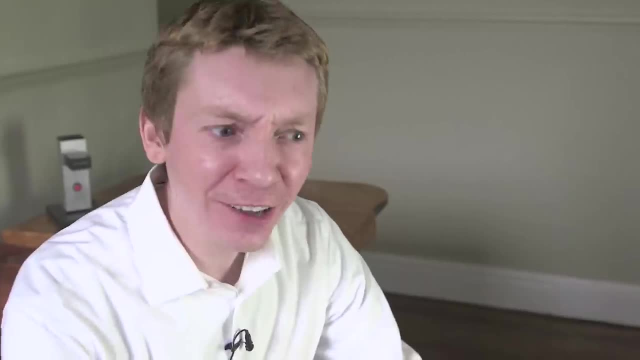 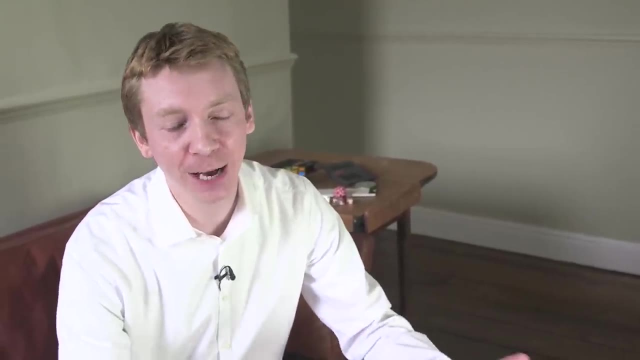 And you can do that, And you can actually do that using his own formula. So these are not particularly easy to calculate, but the largest value we've calculated so far is something around 100 million million million. So it's 20 zeros, a massive number.